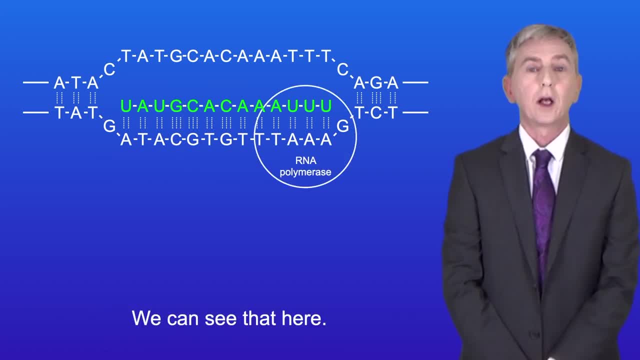 the RNA nucleotides by forming phosphodiester bonds, and we can see that here The enzymes continue making their way along the DNA until they reach the end of the gene. So we've now produced a strand of messenger RNA. Now I just want to mention a quick point here. If you look at the messenger, 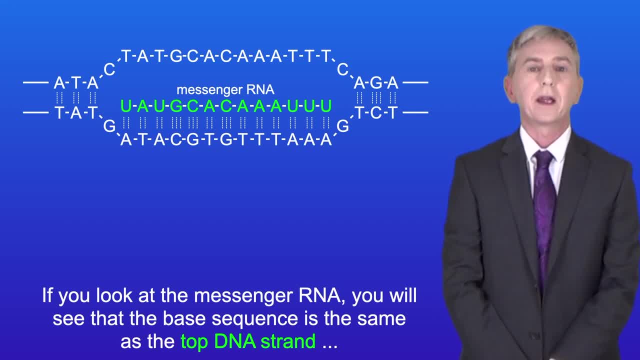 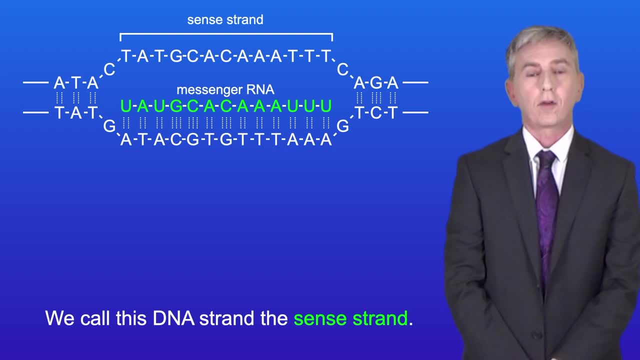 RNA, you'll see that the base sequence is the same as the top DNA strand, except the thiamine has been replaced by uracil. We call this DNA strand the Sens strand. The mRNA is complementary to the other DNA strand and we call this that In this particular case. here we've got the DNA few for action and so I'm just going to tougher do this in the handle. 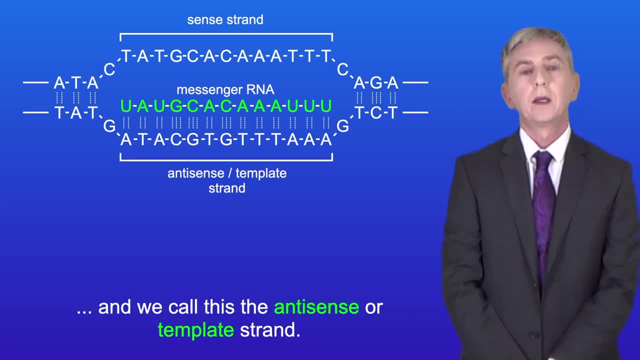 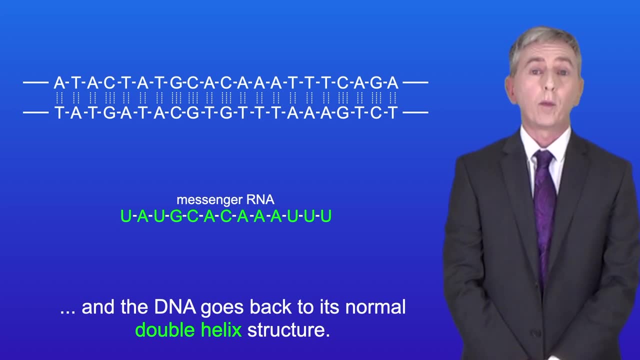 We call this the antisense or template strand. Now, once the mRNA has been synthesised, the RNA polymerase detaches from the DNA and the DNA goes back to its normal double helix structure. At this stage, the mRNA now moves out of the nucleus through a nuclear pore. 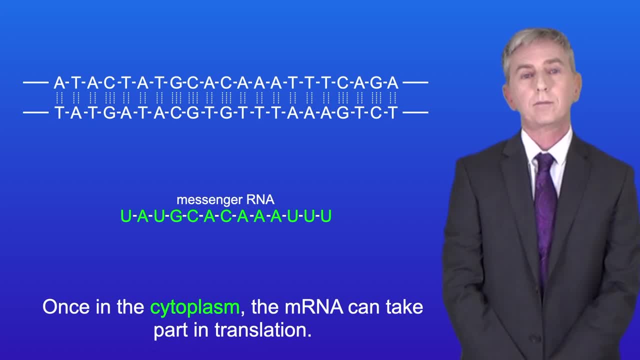 Once in the cytoplasm, the mRNA can take part in translation. Now I should just point out that the mRNA I'm showing you here is much shorter than they normally are. Most mRNA molecules are hundreds of nucleotides long. OK, in the next section we're going to look at the role of RNA splicing, and this applies. 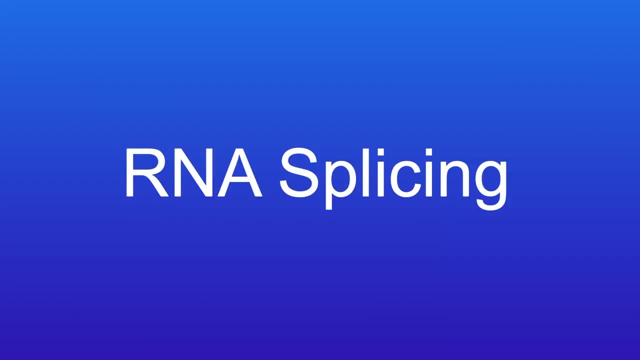 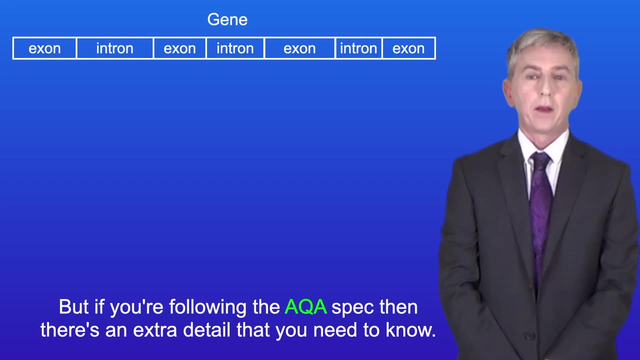 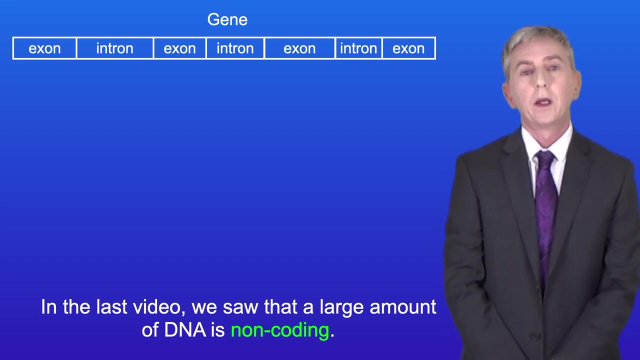 to students following the AQA spec. OK, so we've seen how a messenger RNA molecule is produced, but if you're following the AQA spec, then there's an extra detail that you need to know. In the last video, we saw that a large amount of DNA is non-coding. 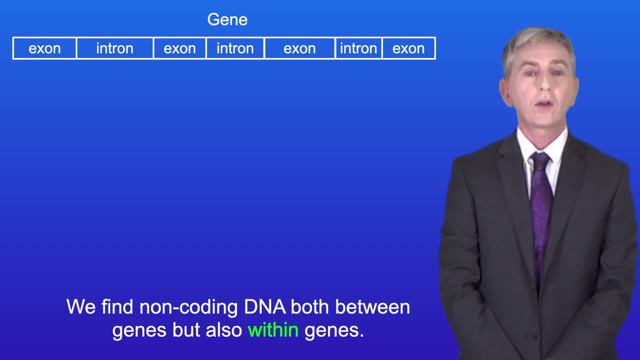 We find non-coding DNA both between genes, but also within genes. I'm showing you the structure of a gene here. Non-coding regions within a gene are called introns, while the coding regions are called exons, And in humans, many genes contain a large number of introns. 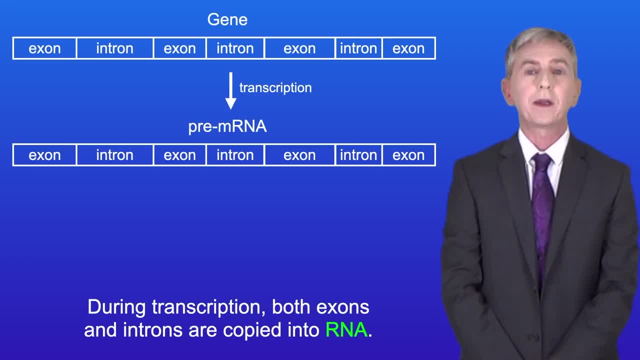 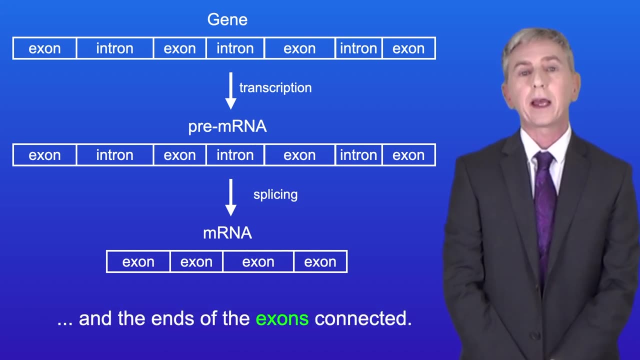 Now, during transcription, both exons and introns are copied into RNA, So that means that the RNA contains non-coding regions. Scientists call this pre-mRNA. Once the pre-mRNA is formed, The introns are then removed and the ends of the exons connected.